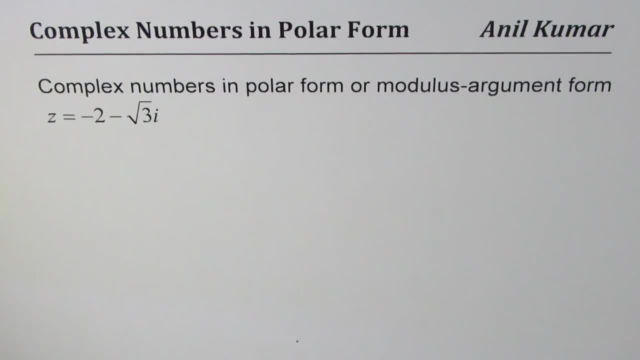 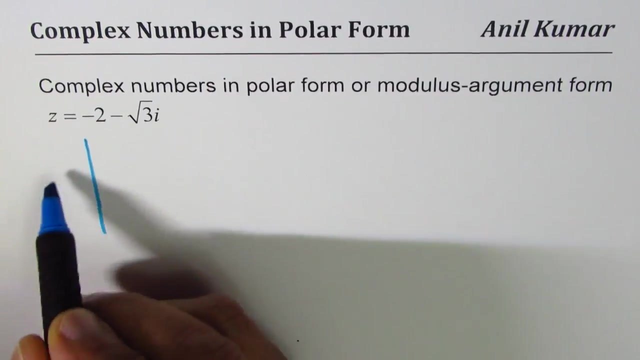 I am Adil Kumar, sharing with you a technique of writing complex numbers in polar form. In this particular example, the complex number is minus 2, minus square root 3i. Both are negative. so both are negative means we are in coordinate 3. Perfect. 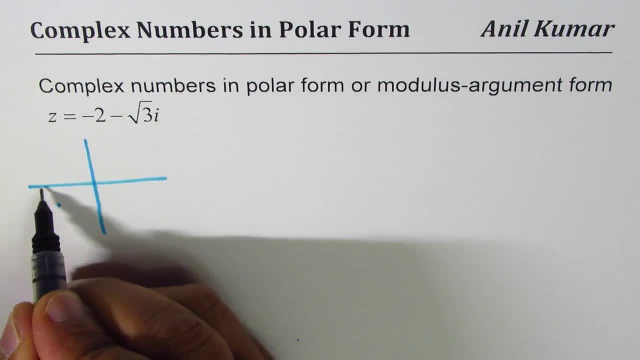 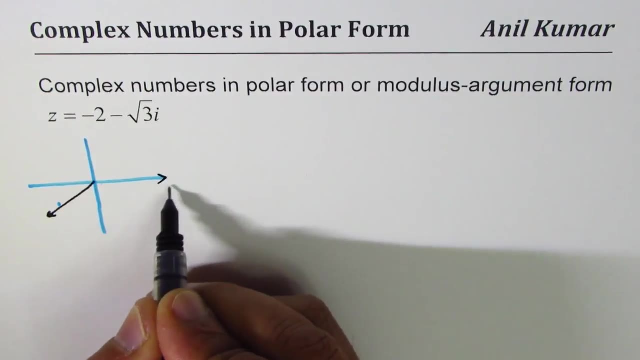 So let us get into it. Minus 2 means 2 units to the left. minus square root 3 means square root 3 down right. So somewhere kind of like this will be our complex number represented, where this is positive real numbers on the polar axis. and here we have imaginary numbers, correct? Let us say this: 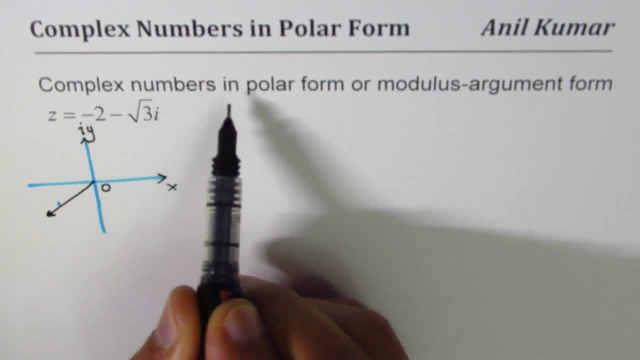 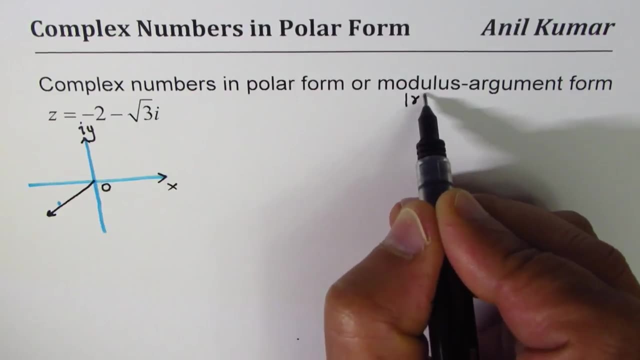 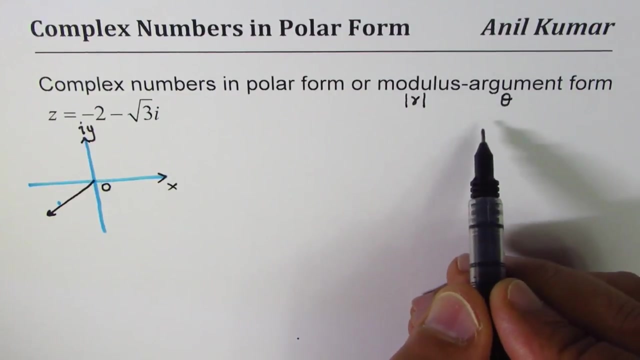 is O. Now when we say that the complex number in polar form, which is also modulus argument form, modulus is r. the magnitude Argument is theta, the angle. Most of the time we work in radians. Now some students. 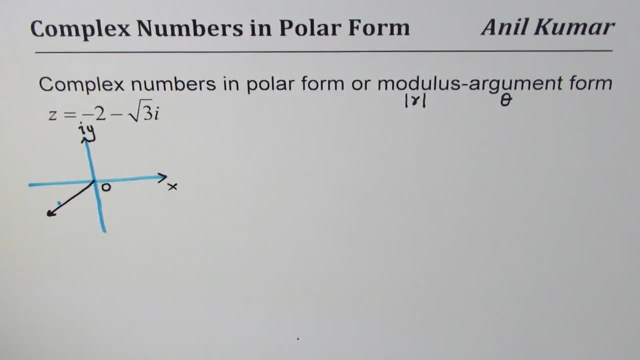 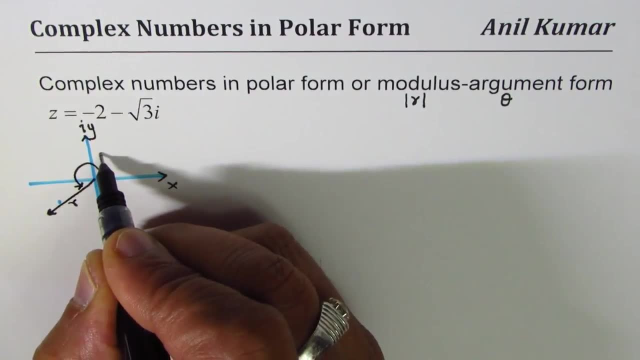 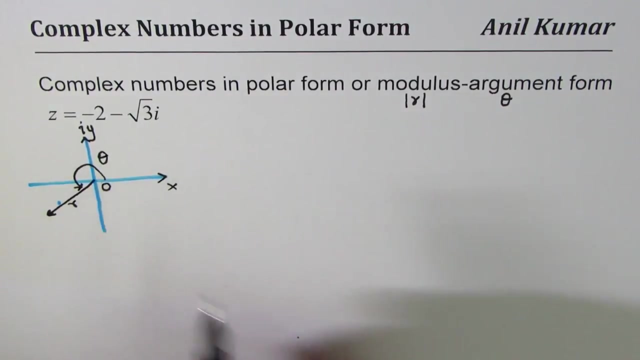 work in degrees. Both is okay, right. Both are fine, right. So r is this length and theta is this angle. Let us take it positive for the time being. So that is the situation. Let us see how to do it. General method is: normally we say z is. 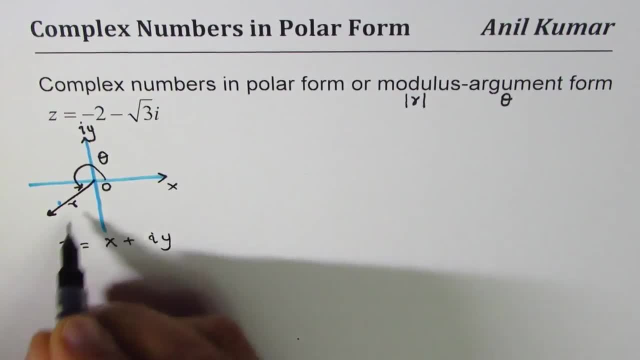 x plus i, y, So r will be using Pythagorean theorem, x square plus y square, square root and theta you can find using tan theta equals to y over x And of course with tan theta you have two options. So better thing is first to find acute angle right tan alpha with positive values of y over x. 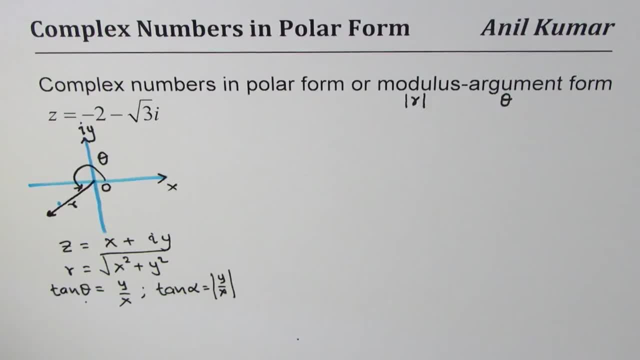 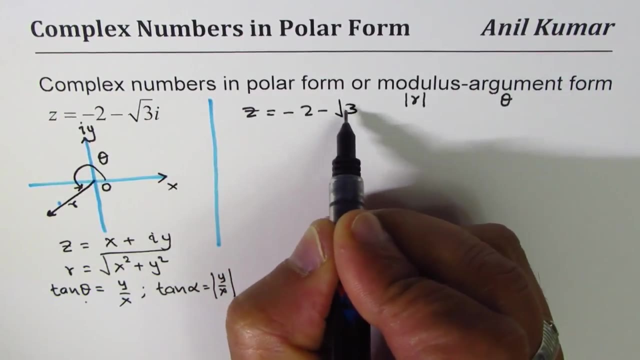 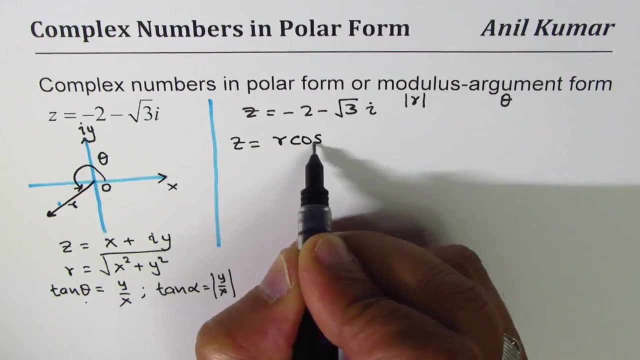 And then figure out theta, Is it okay? So that is a strategy to work with. So let us begin. We need to write the complex number which is: z equals to minus 2, minus square root, 3, i in polar form, that is to say, as r cos theta plus i r sin theta right, Since r is. 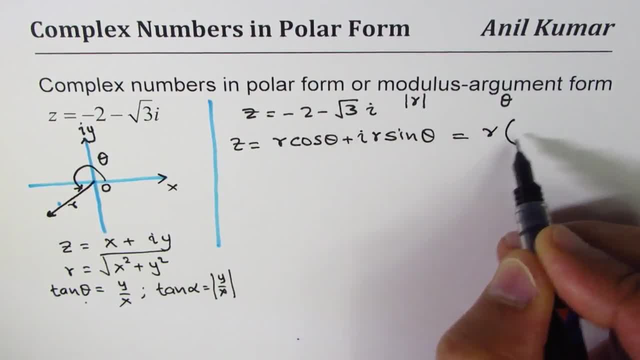 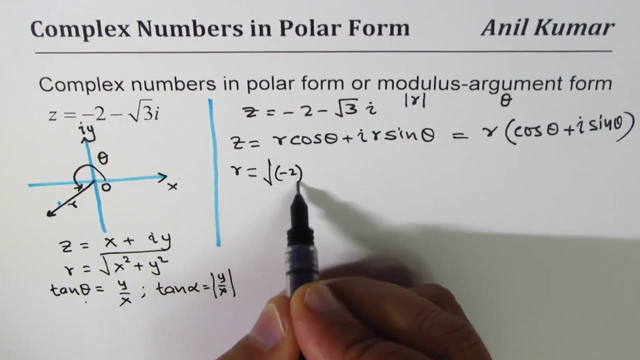 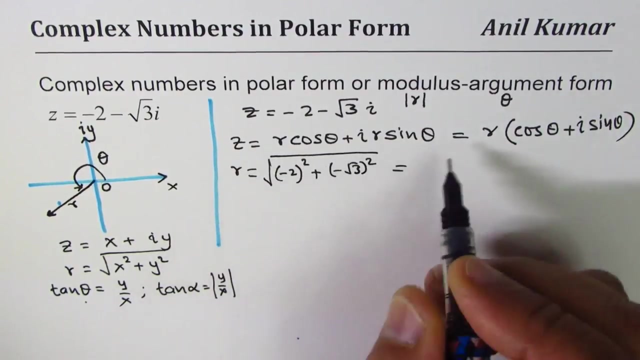 common. it is better to write r as a common factor. It is always written like this: only Cos theta plus. i sin theta, right. Okay, So let us find r first. R in this case x is minus 2.. So it is minus 2 square plus, minus square root, 3 square Square root, And that gives us square root of. 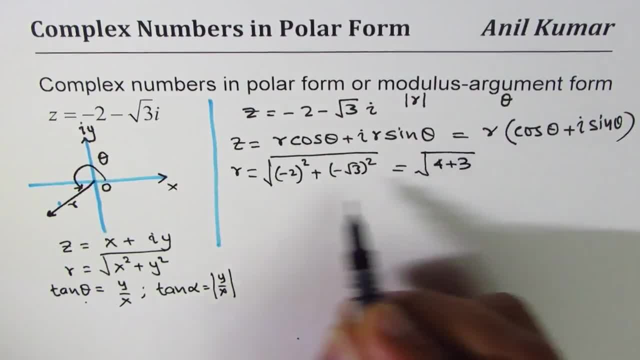 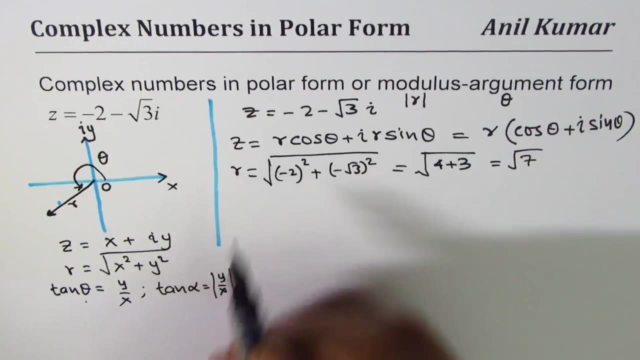 4 plus 3, correct, 4 plus 3 is 7.. So square root of 7 we get- That's the value of r, always taken positive, right? I don't have to write modulus and all, because square root gives you positive values. 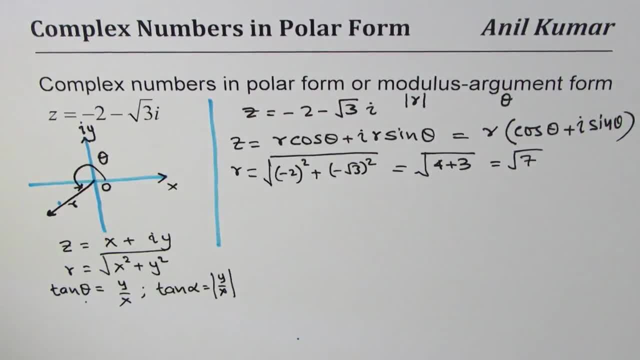 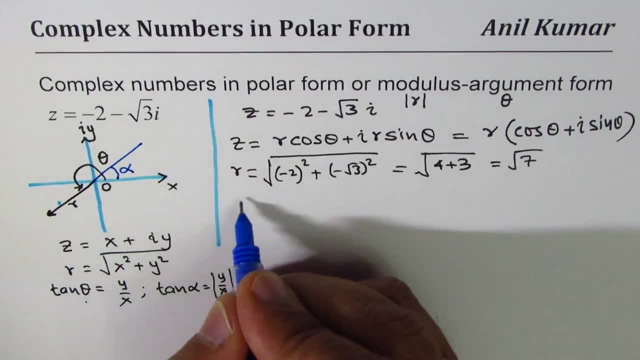 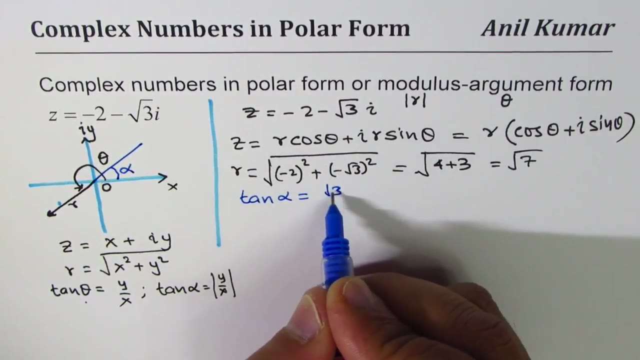 Okay, Now let's find theta. As we have always said, it's better to find the related acute angle alpha first. So let's find alpha first. So tan alpha is equal to sine over cos, So square root 3 over 2. And that gives you alpha as equal to. well, that is a special triangle. 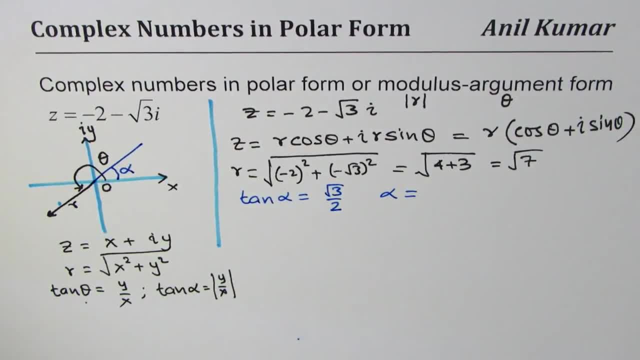 correct. So let me sketch one, and then we'll figure it out, the value itself. So we can use calculator also, no problems. Well, sometimes you have values where special values are equal to special values. So let's find alpha first. So tan alpha is equal to. 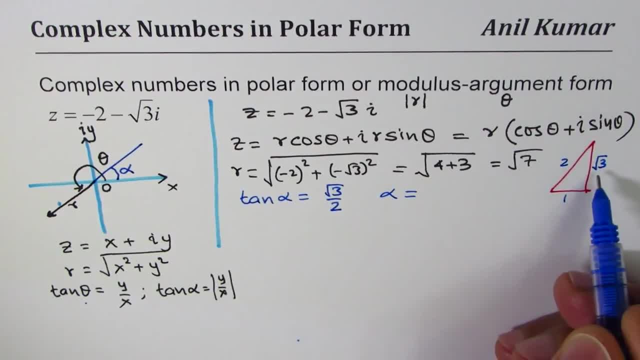 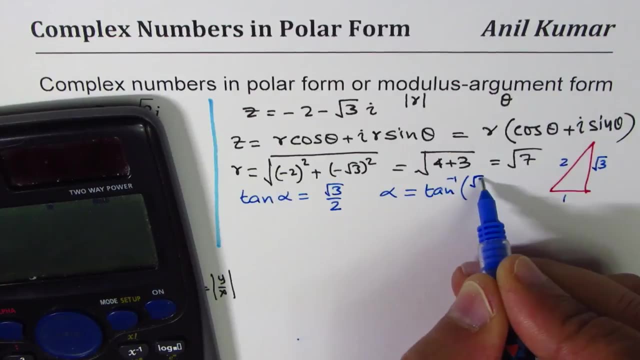 better to use your knowledge. Square root 3 over 2,. I'm sorry That doesn't work. Square root 3 over 2.. So let's use calculator. So alpha is tan inverse, Okay, Tan inverse. square root 3 over 2,. 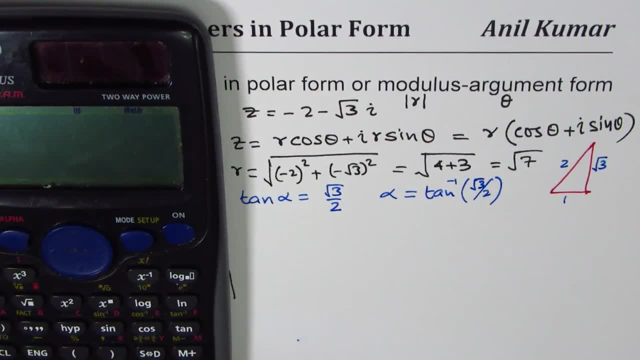 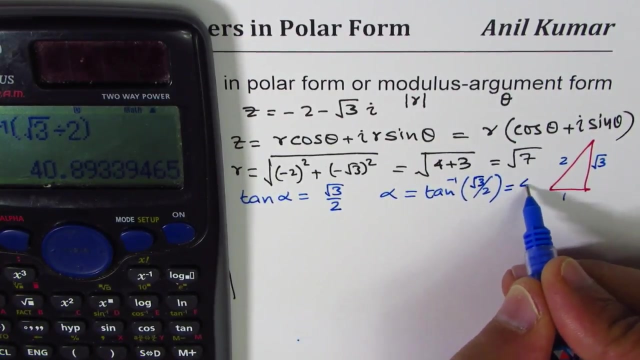 correct. So we do shift tan inverse within bracket. We have square root 3.. And then we'll divide this by 2.. You could have put slash and say equal to. So this seems to be in degrees, So we'll just round this to 41 degrees. Okay, It says 40.89.. So I'm rounding it. 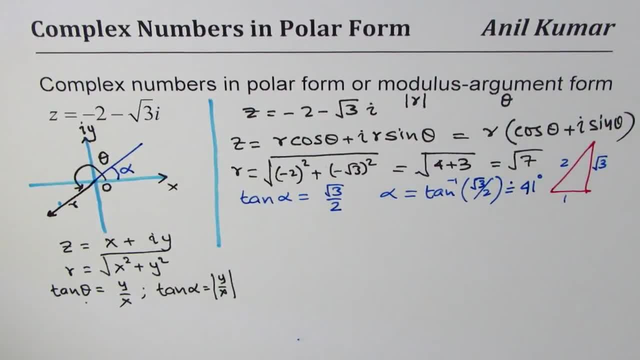 to 41 degrees. Let me write approximately. So we got alpha as 41 degrees, right. You could change the mode and write Answer in radians. Radiance is better, But most of my students in grade 11, they haven't learned.